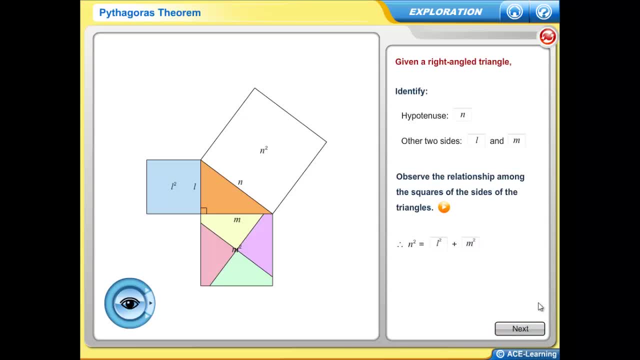 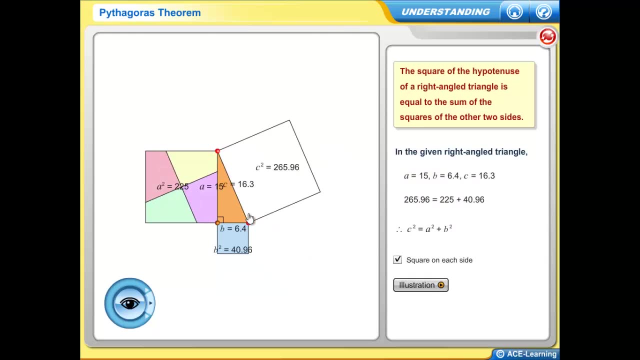 In the Understanding section we give students lots of room to test out what they have discovered earlier under exploration. For example, they can resize the given figure, toggle the vertices, rotate the figure, view the animation, etc. Next they are prompted to proceed to Application. 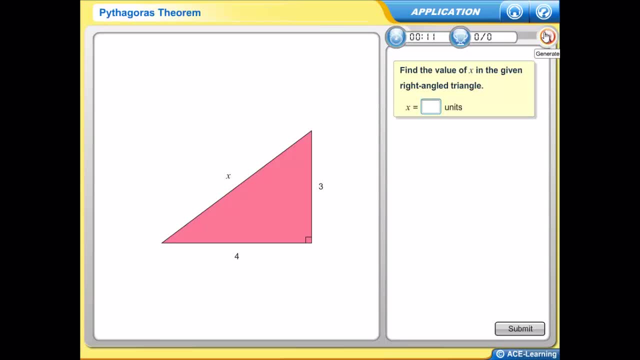 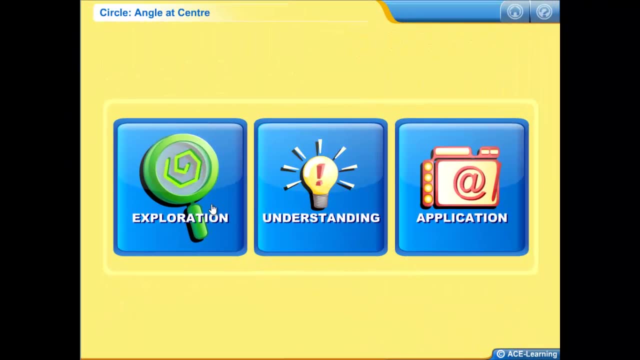 Under Application. randomly generated exercises test whether a student has understood the concept of that application. In the Exploration section they are asked to find out whether they have understood the concept of that application. Now let's take a look at one of the circle properties. angle at center. 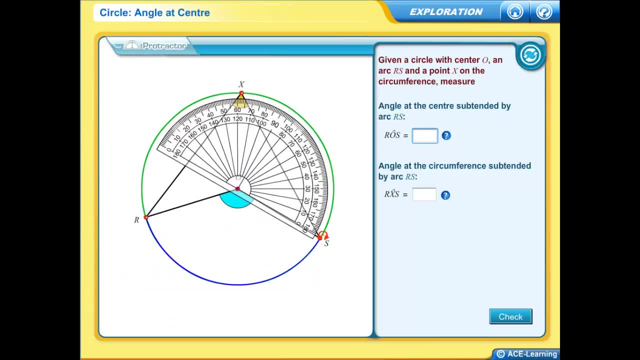 In the Exploration section, a protractor is provided to help them in the exploration. A zoom feature is also provided for a magnified view. So students make use of the protractor to find the measurements of the angles, input the answers and view the animation to observe the relationship. 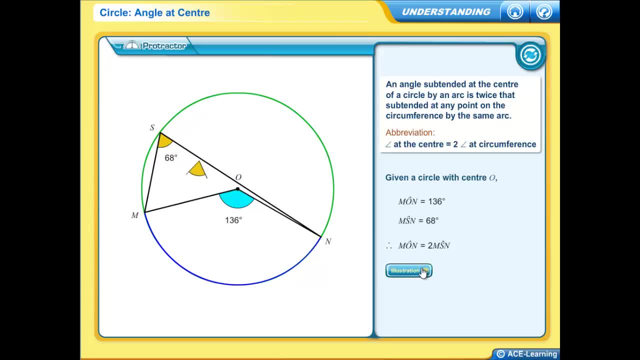 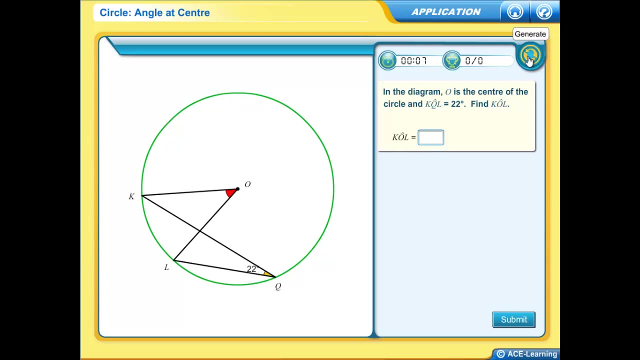 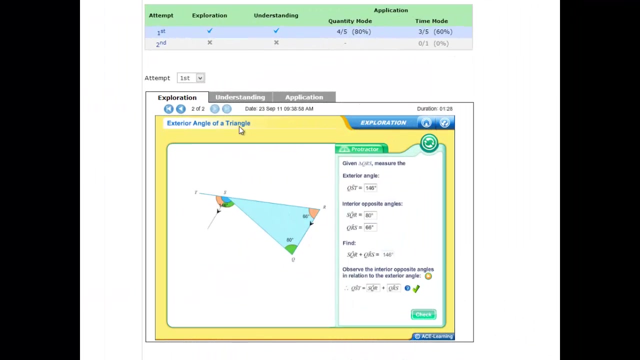 In the Understanding section, students are prompted to look at various cases and view the animation each time to see if the property still applies in each of those cases, After which they are prompted to proceed to Application. Now here comes the best part- Print screens are done- of the student's exploratory journey. 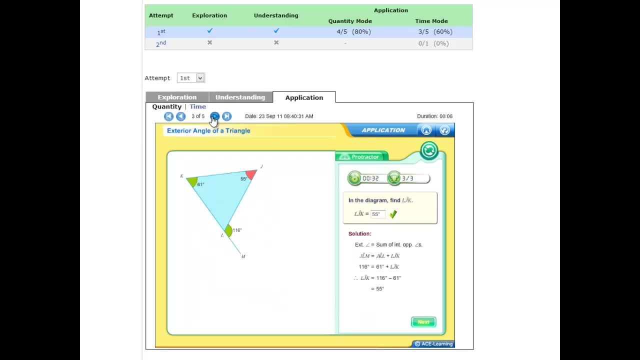 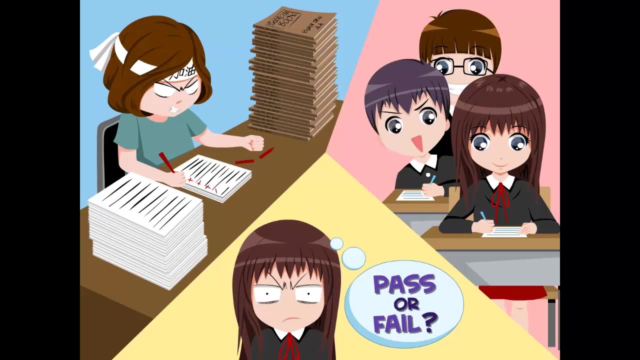 and reflected in the report. We know the importance of practice when it comes to mastering math topics. If homework is given, marking has to be done. Students also won't know whether their answers are correct until they have received the marked homework. Is there an alternative solution? 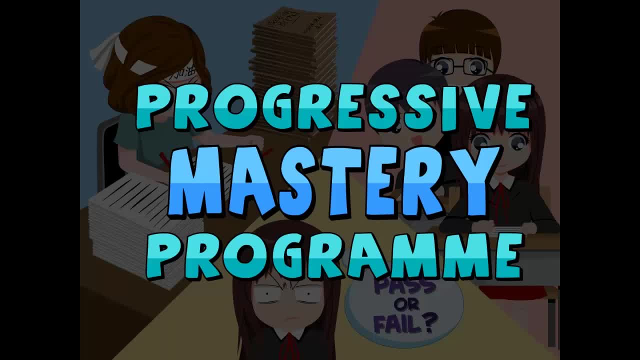 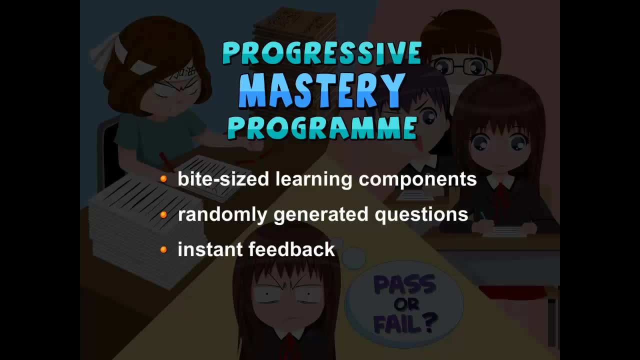 Yes, there is The Progressive Mastery Program, or PMP for short. In the PMP, topics are broken down into three parts. Topics are broken down into bite-sized learning components to pace students' learning. Questions are randomly generated to resolve the problem of. 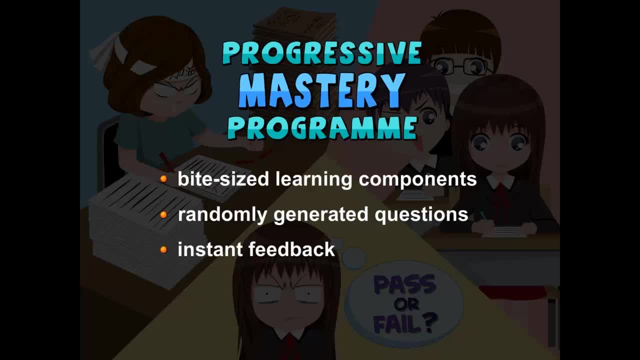 one student doing the homework. the rest of the class copy Instant feedback after each solution is submitted or after each step for guided PMPs. Let's take a look at how we designed this learning program. This topic is Solving Linear Equations. 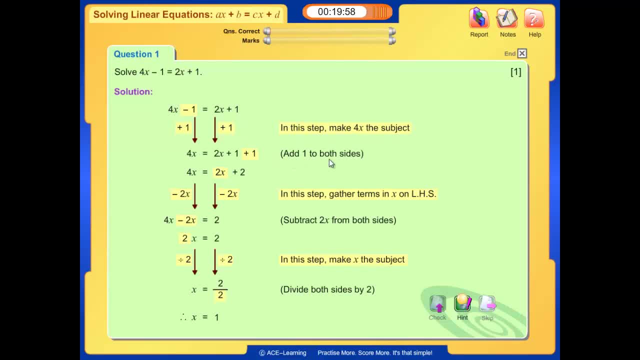 We have students who are so weak in this topic that they don't even know when to start. Well, not to worry, let the system guide them. If they are unsure and need further help, click on Hint. Step by step, the system takes them through the solution. 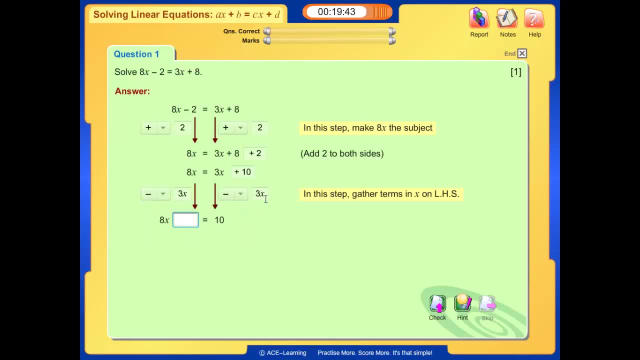 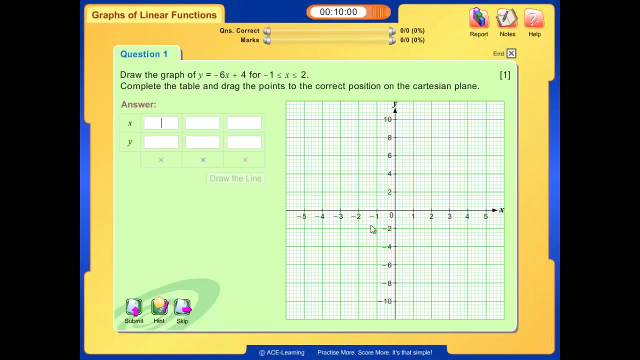 Line by line. the system auto-marks the input. If they make a mistake, they are not allowed to continue until they have corrected it. Now let's take a look at another topic: graphs of linear functions. To begin, select a range of values. 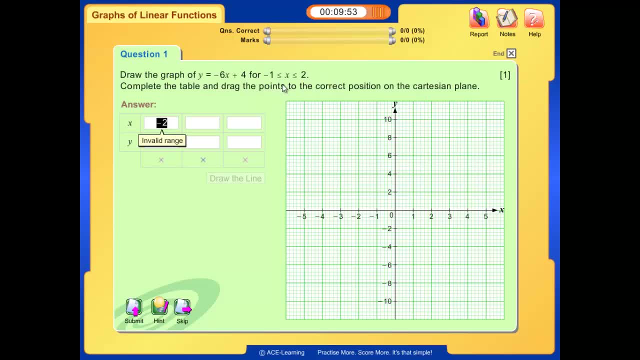 Oops, invalid range. The student has failed to notice that a range of values has been given. This is a common problem, So with this PMP, the student learns to read the question carefully. Now let's keep the x values within the given range. 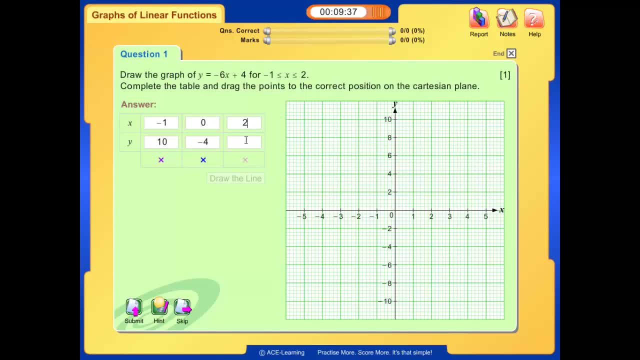 Calculate the y values. As each y value is keyed in, a small cross appears. Ah, notice that there is a mistake made. We'll see how the system prompts the student later. Let's position the points first. Oops, incorrect position. 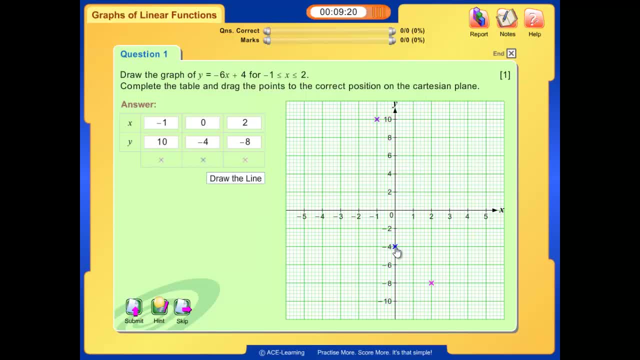 Try again. Next, draw the line. The line is not straight. This is a linear graph, so the line drawn should be straight. Of course, the student can go ahead and submit the answer, but he or she can see that there is a mistake somewhere. 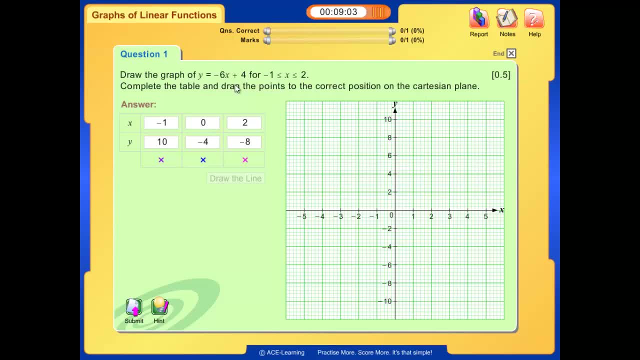 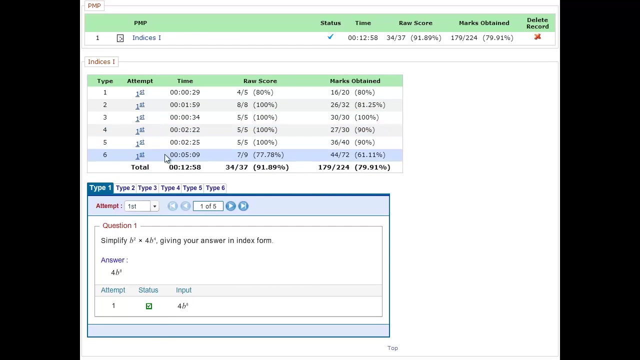 So retrace the steps, Identify the problem, Correct it, Try again, And there we have the required linear graph. Next we'll look at how comprehensive our reports are. for the PMP, This is an individual student's report. The result for each level and type of question for the topic is reflected in the report. 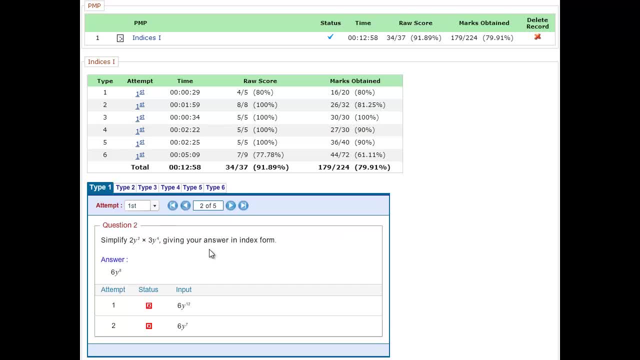 As mentioned, each student is given a unique set of exercises, so the report should be able to reflect that This question is unique to this student. Now here comes the best part. Every attempts input is reflected in the report. This is a very good diagnostic tool. 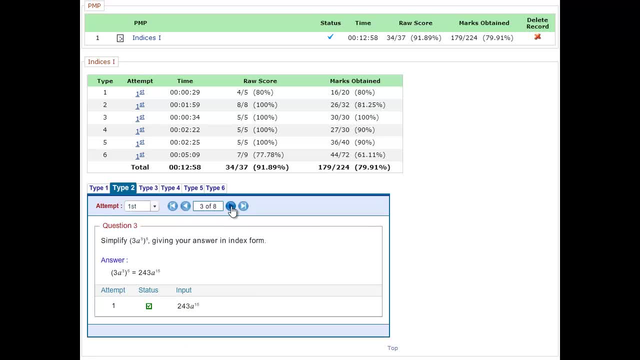 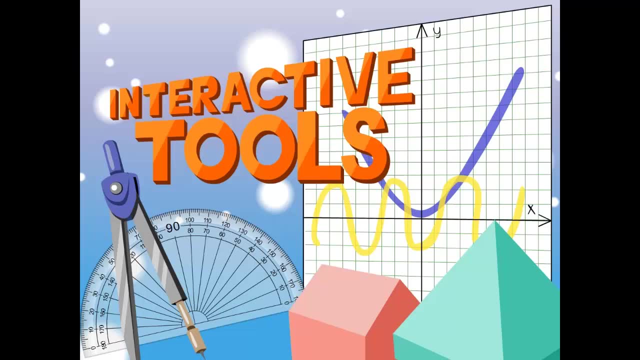 From each attempts input, one is able to know the area of the student's weakness in the topic. Interactive tools are a great medium for understanding math concepts. Let's take a look at two unique tools: All-in-one grapher and 3D tool. 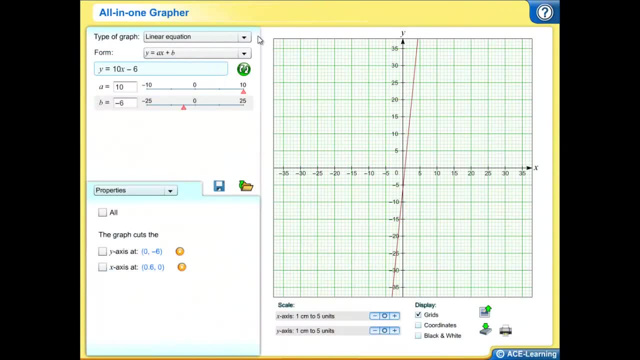 As the name suggests, the all-in-one grapher enables one to plot multiple function graphs on the same Cartesian plane. Let's demonstrate the power and ease of using this tool by plotting a quadratic graph. First select the type of graph, Then its form. 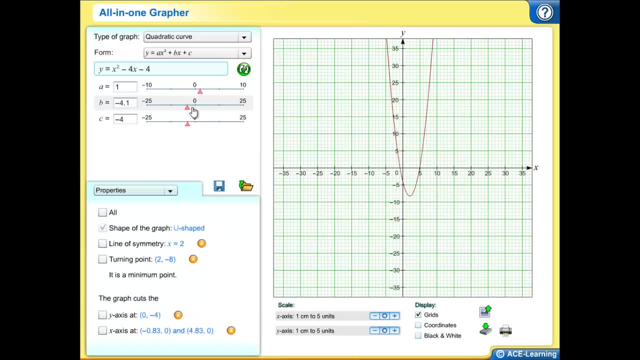 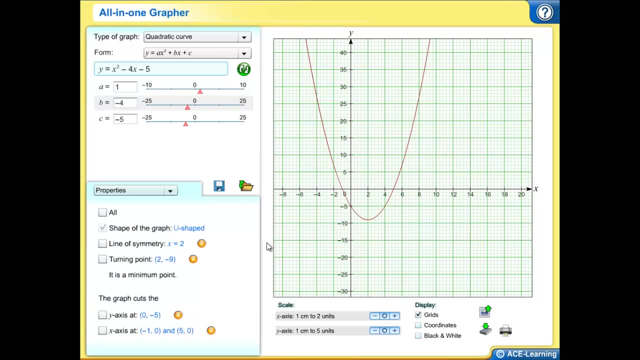 Finally, the coefficients and constants. You may key in the figures in the boxes or use the slide rule. Here's how you can adjust the scale. Voila, the quadratic graph is done. Now let's take a look at the unique features of this grapher. 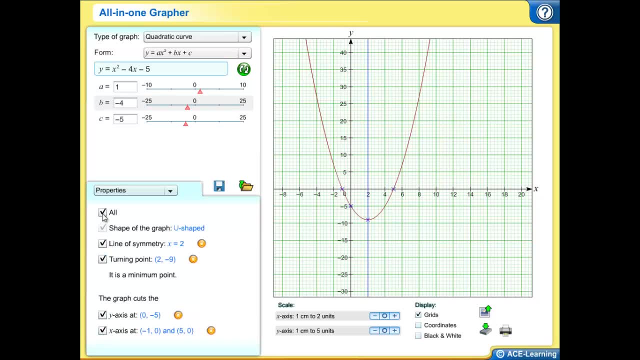 You can select the properties you want reflected on the graph If you want to view the data table or XY values here it is Solution to the function Formula to use Gradients. No problem. Now let's try to plot a trigonometry function using the same stamps. 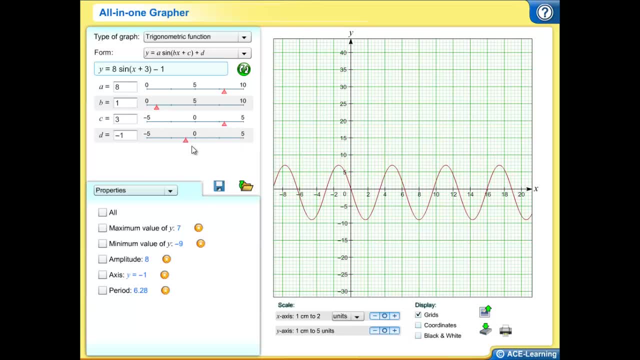 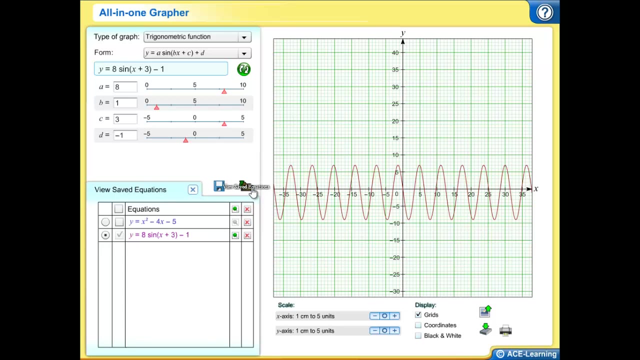 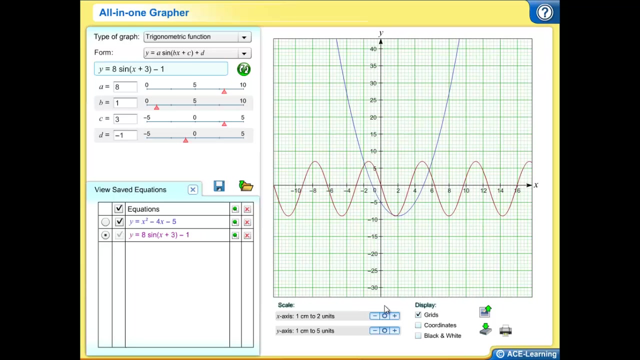 Let's take a look at some of its properties. Maybe gradients too. Shall we overlay some graphs and design a simple assignment? Here we go. Now we have two graphs on the same Cartesian plane. Let's get rid of the grid lines and have a sketch instead. 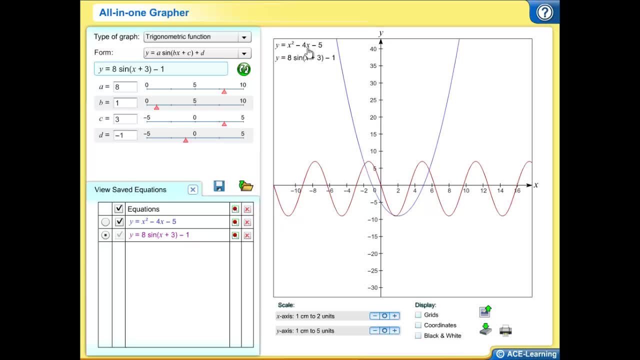 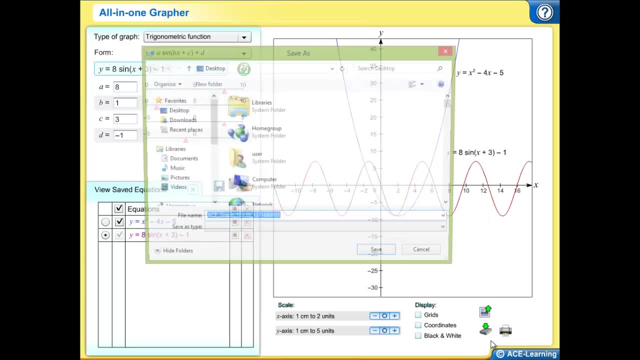 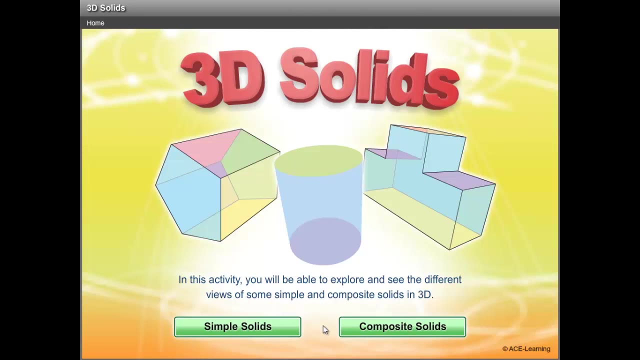 Now let's have the equations presented As an assignment. the students are required to match the equation to the graph. The graph can also be downloaded and attached to documents. Now let's take a look at the 3D tools. Let's begin with the first 3D tool for simple and composite solids. 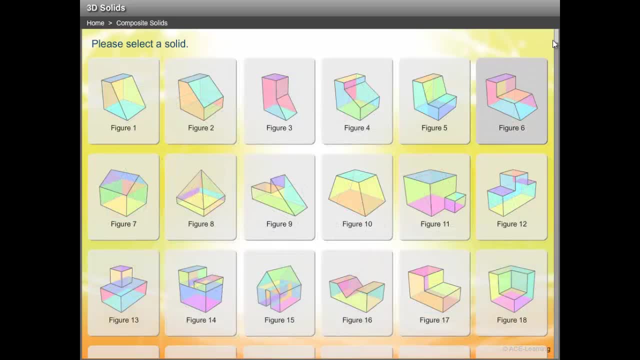 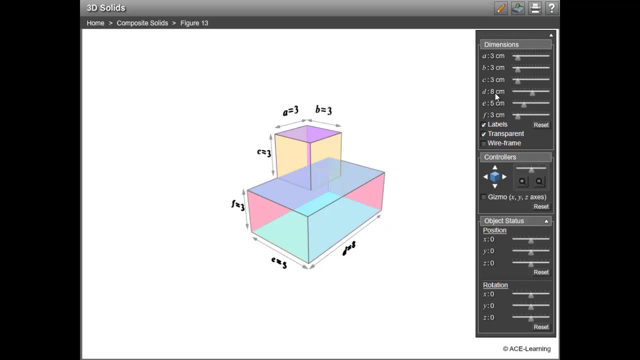 Here is a ready pool of simple solids And a pool of composite solids To begin select a solid. You can modify the solid any way you want it, rotate it, even magnify it. If you need a plan view, side or front elevation view, no problem. 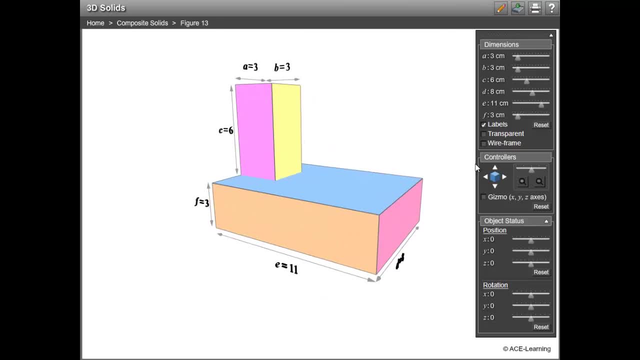 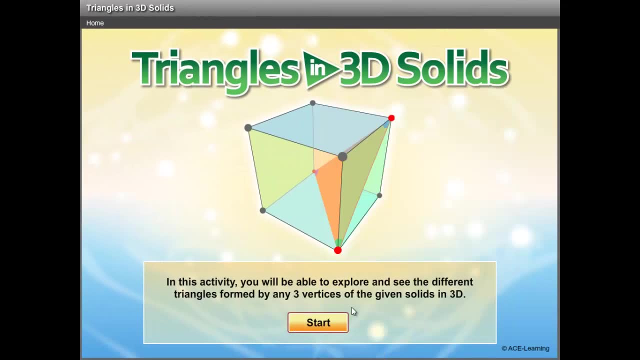 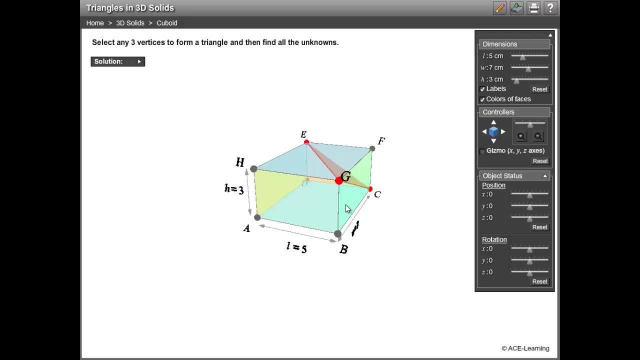 If a wireframe is what you desire, by all means. Now let's take a look at the 3D tool for triangles in 3D To begin, select a solid. Now let's have the triangle in the solid. If you want the reference triangle to stand out, no problem. 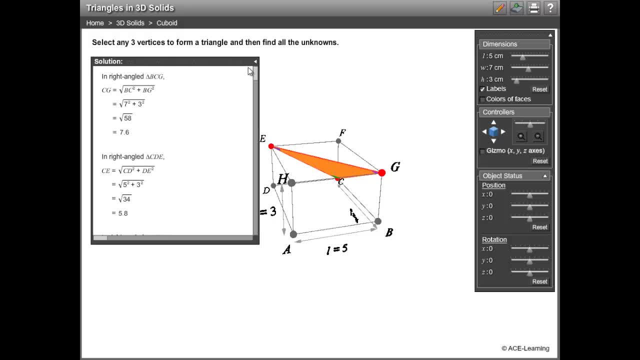 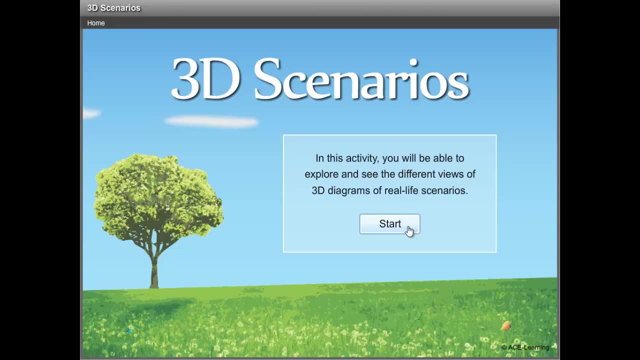 Solutions are also provided. Notice how the values in the solution changes when the object is modified. Now the third 3D tool is for 3D diagrams of various shapes, 3D diagrams of real-life scenarios. Let's select a scenario. 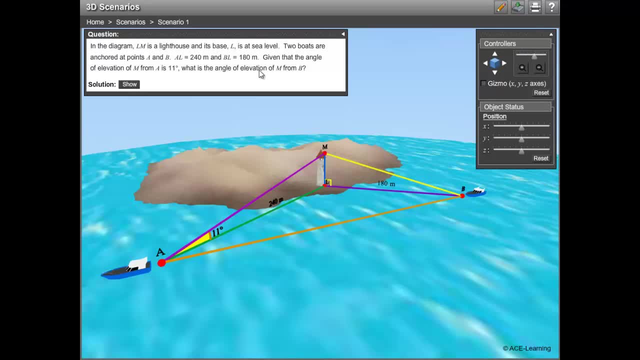 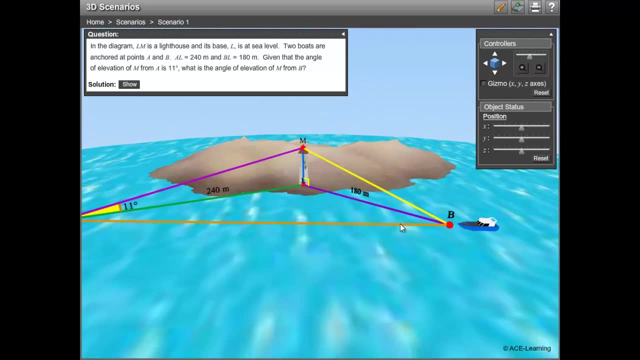 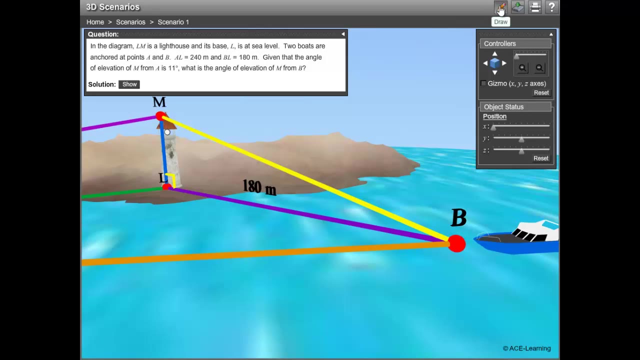 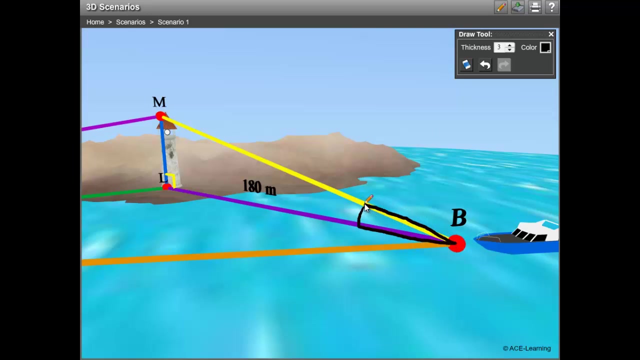 First view the problem. We are to find the angle of elevation of M from B. Next, locate the triangle where the required angle is Right. it is in this triangle And this is the required angle. Now for the solution. Here there is a unique feature which other systems do not have. 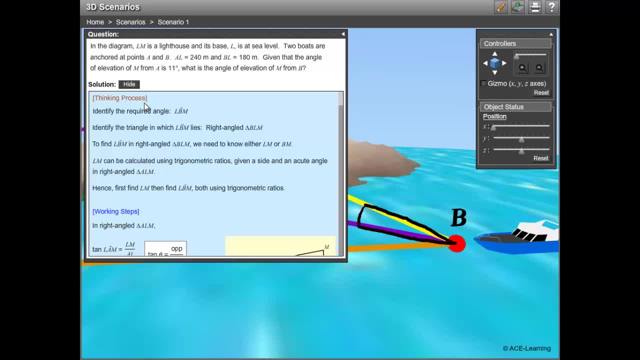 Thinking process. Before any attempts on problem solving, the thinking process is crucial. Students need to understand the problem, identify what they are required to find and manipulate the given information to solve the problem. Are you preparing for a national examination and want concise notes with ample practice questions?